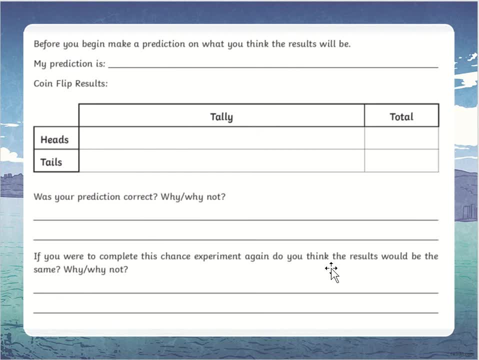 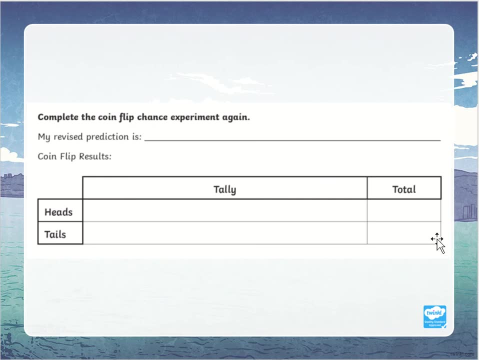 to complete this chance experiment again. do you think the results would be the same? so you put in yes, no because okay, and then you're going to do it again. so redo your prediction and then do it again, put in your tally, put in your total, and then you're going to answer these questions. 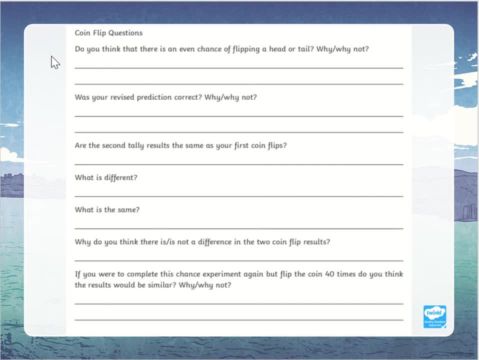 do you think there is an even chance of flipping a head or tail? why or why not? was your revised prediction correct? why or why not? are the second tally results the same as your first coin flips? what was different? what was the same? why do you think there is or is not a difference in the two? 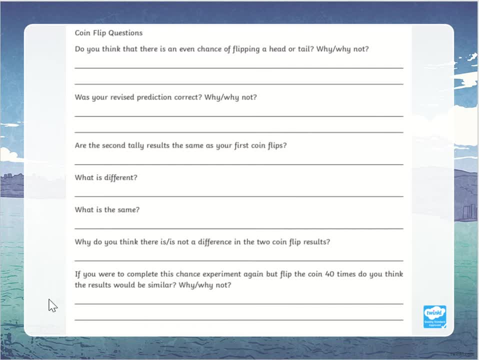 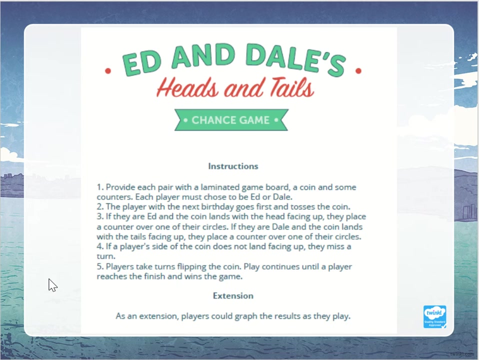 coin flip results. if you were able to complete this chance experiment again, but you flipped the coin 40 times, do you think the results would be similar? why or why not? okay, if you'd like to do a chance game with another player, then you definitely can. okay, so what you're going to do is: 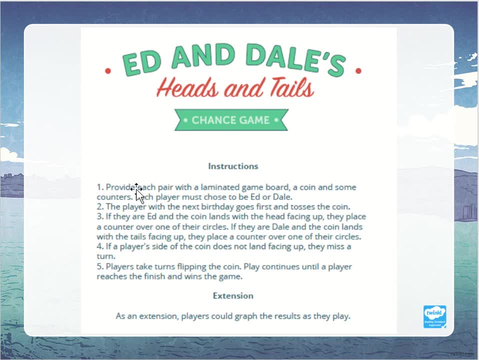 to um pick whether you want to be ed or dale. okay, so there are two characters in here, so the player with the next birthday, they are going to go first. they toss a coin. if it's ed and the coin lands with the head facing up, then you can place a counter to cover one of 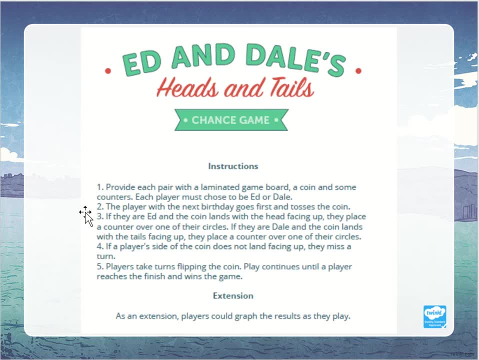 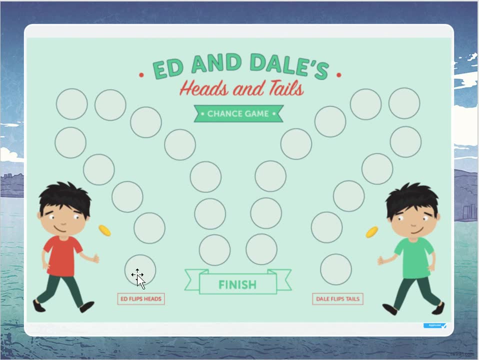 your circles. okay, so if you are dale and the coin lands with tails up, then you can place a counter circle. so this is what it looks like. so every time, if you choose to be ed, then every time you get heads, you can put a counter on the circle if you like, or you can like cross it off, etc. okay, 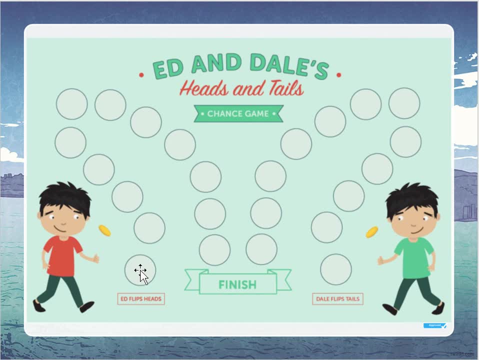 so this is: if you want to play a game with someone else, um, and then we have dale. so if you choose to be the character dale, and every time you get tails, then you get to cross one circle off or you get to put a counter on there. so the whole aim of the game is to see who gets to go to the. 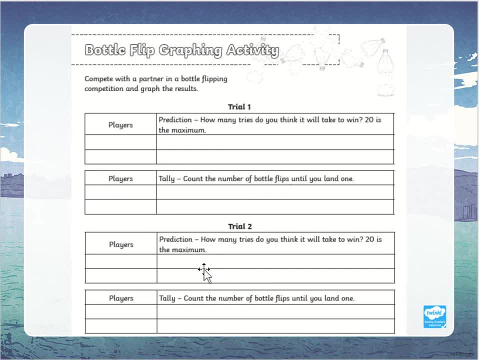 finish line first. what you can also do is do a bottle flipping activity as well, so you can um pick your if you have multiple players, or you can do this on your own as well. okay, so you put the players names down, so, um, there are. so you and a partner can do this, or you can do this on your own. 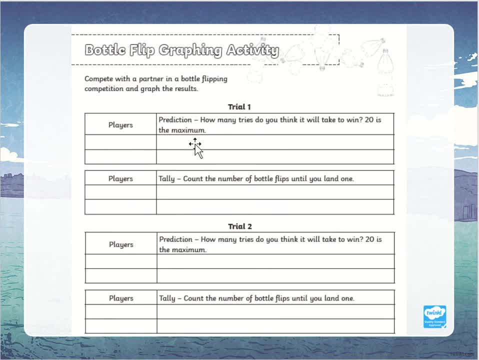 so there are. so you and a partner can do this, or you can do this on your own. you put the names of the players here, you predict how many tries do you think it will take to win the bottle flipping competition? so 20 is the maximum. so have a prediction, see if you. 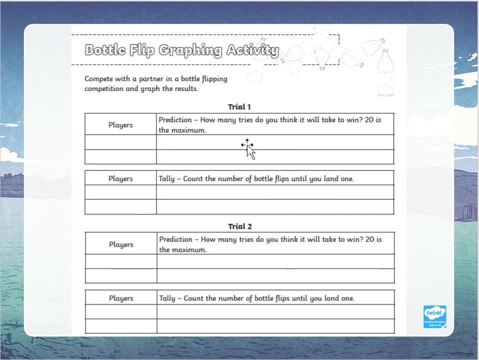 can guess how many times, how many times you can bottle flip, and then you're going to tally, so you're going to count the number of body bottle flips until you land one. so you have to try to predict how many times do you think it will take for you to flip your bottle for it to land, okay, and then you put. 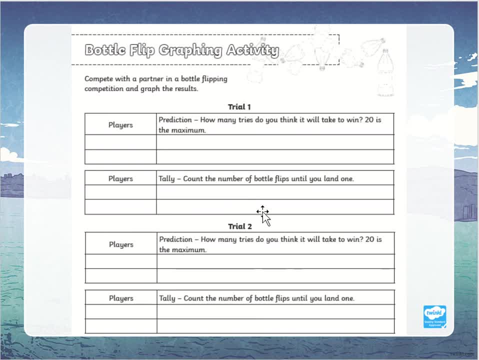 your prediction there and then you actually do the activity. so you flip your bottle, try to flip it as many times as you can until it lands, okay, and then you write the number here and then your partner will also do it. they'll try to flip their bottle over and over again to. 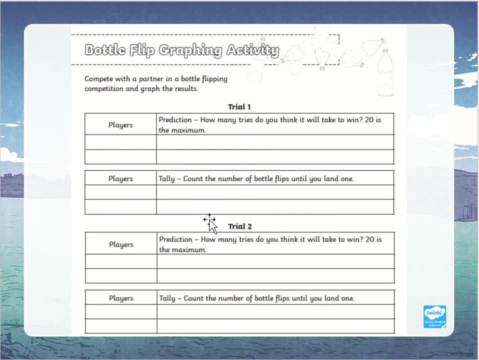 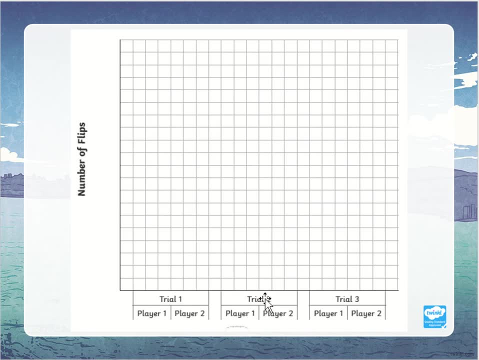 see how many times it will take until it lands, okay. and then you go again, and then you try, try that again and then, after you do that, you can see if you can graph it. so you can graph, you could put numbers on the side of this graph number. 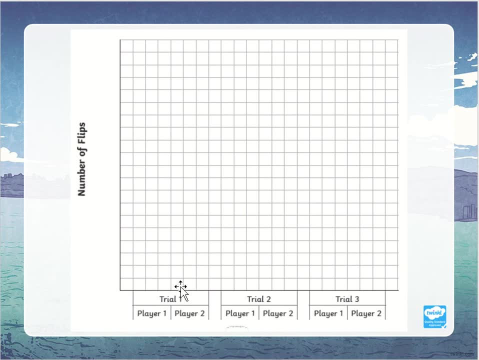 of flips and then you can draw a column graph and draw yeah and graph your.